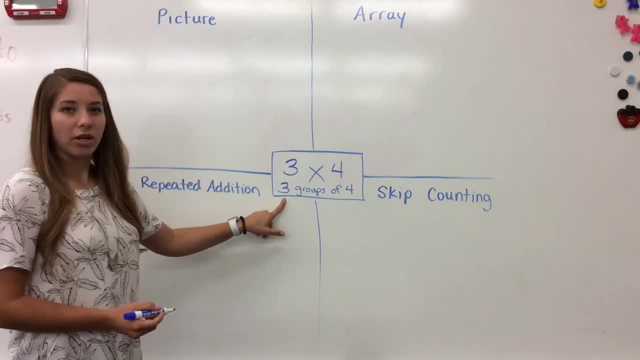 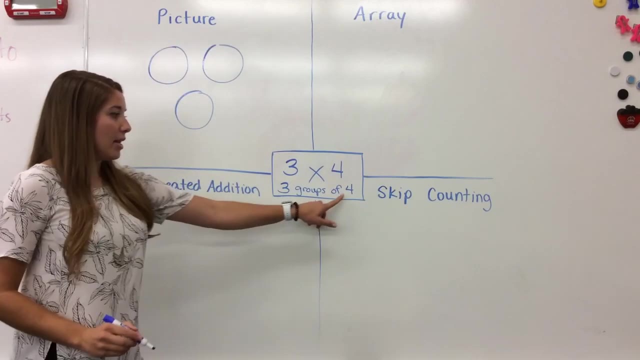 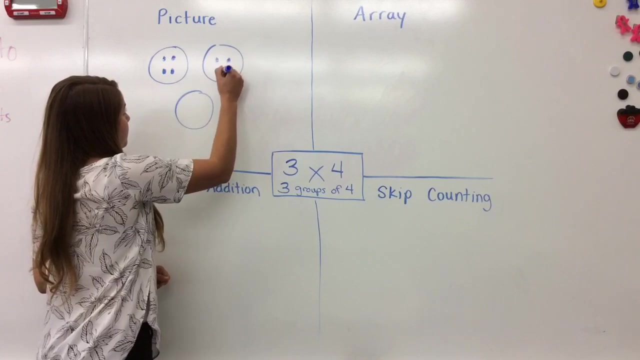 graders is to make a picture. So what I'm going to do is I'm going to start by drawing my three groups And I'm just going to draw three big circles here And then inside each circle I'm going to put four dots: One, two, three, four, Once I have my three groups of four. 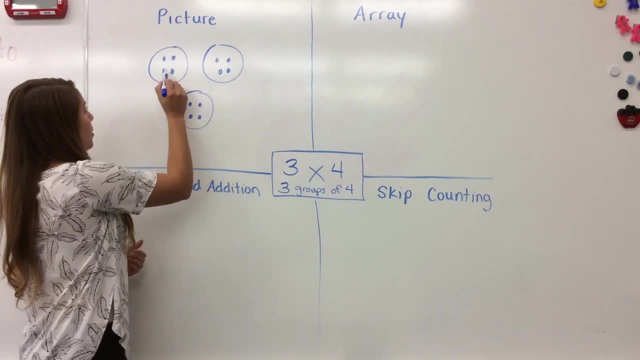 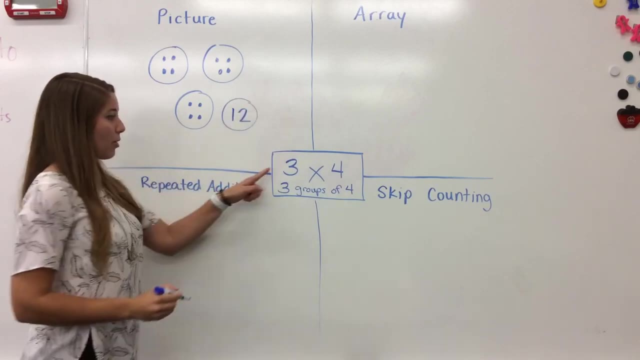 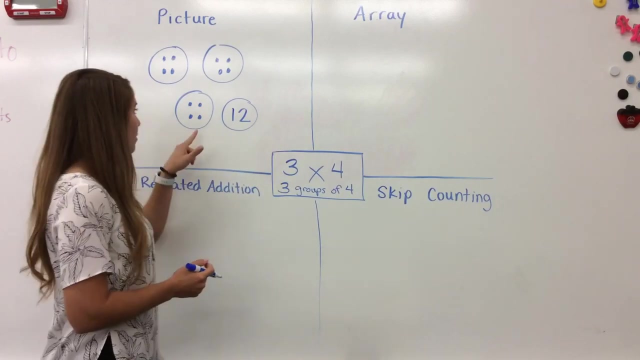 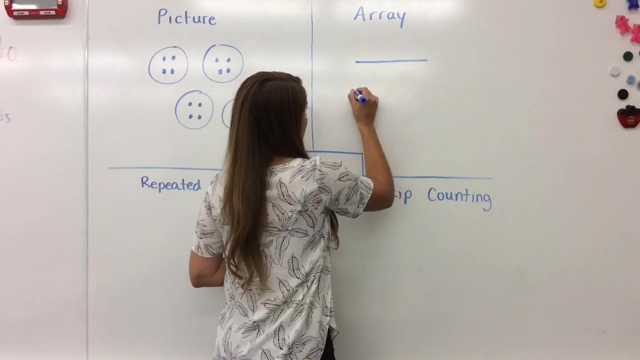 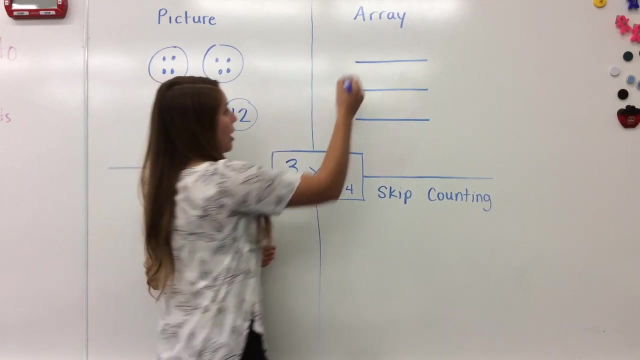 to find my answer. all I need to do is count One, two, three, four, five, six, seven, eight, nine, ten, eleven, twelve. So there is my answer. If I get to the problem three times four using a picture, I get the answer of twelve. Now, an array is very similar to a picture model, but instead of doing three groups as circles, I'm going to do my three groups as rows. So I'm going to draw three lines horizontally across my paper And on each of these rows I'm going to put four objects. I like to use circles. 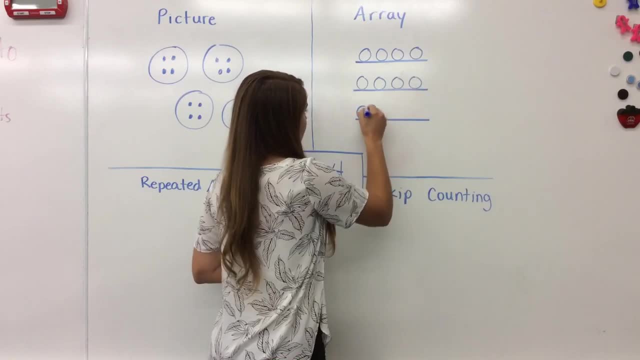 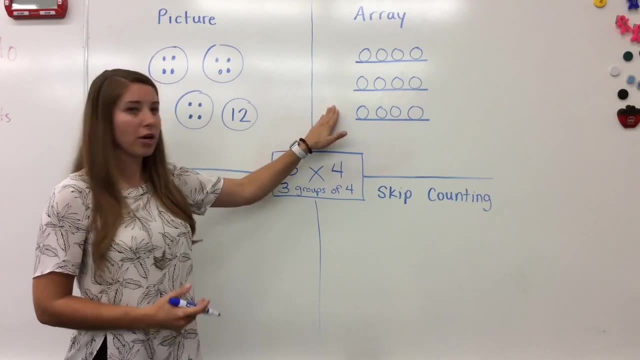 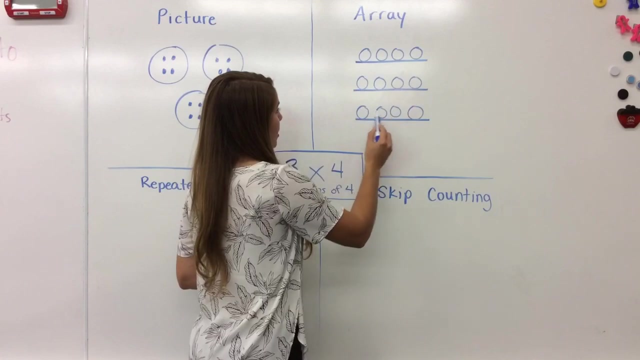 One, two, three, four, And one, two, three, four. Again, I've got my three groups or three rows of four. So to find my total amount I just need to add them up and count them up: One, two, three, four, five, six, seven, eight, nine, ten, eleven, twelve. 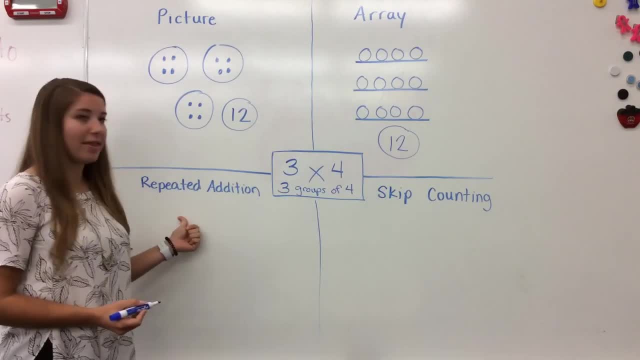 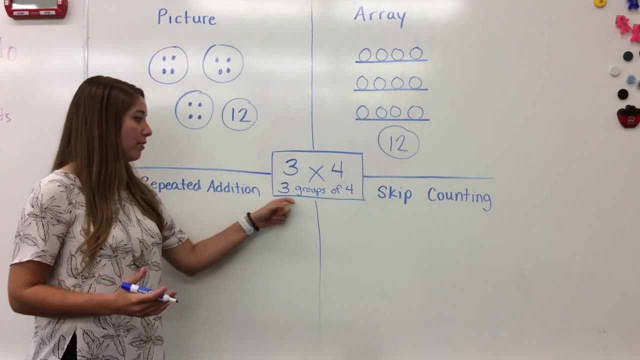 The next strategy that I'm going to show you is repeated addition, And this works again the same way as these other strategies, if I know that multiplication means finding the total amount of equal groups. So what I'm going to do is I'm going to create a group of four. 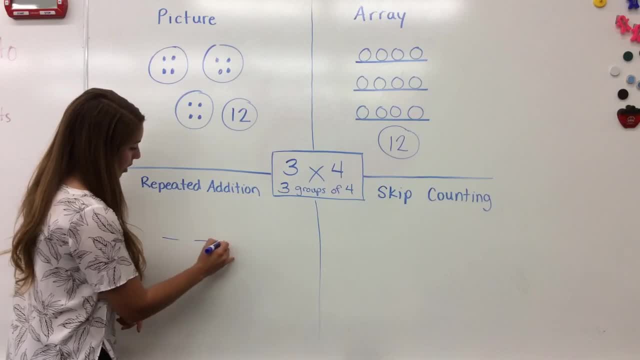 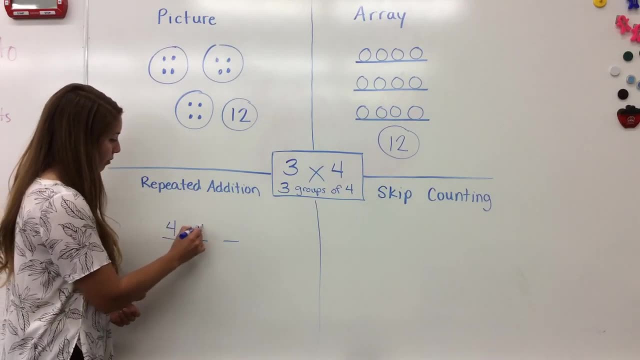 So I'm going to create my three groups by just drawing a little underline- Two and three, And on each of those lines I'm going to put that number four. This time I'm just going to write the number Four, four, four. 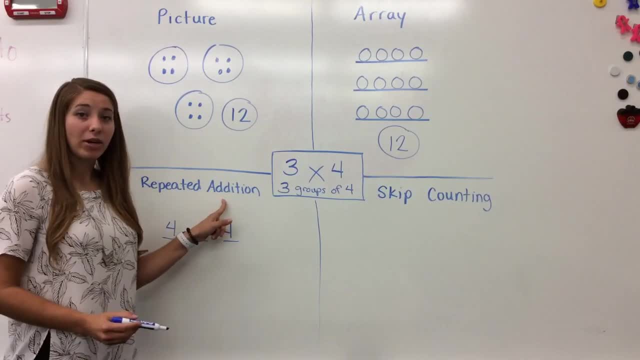 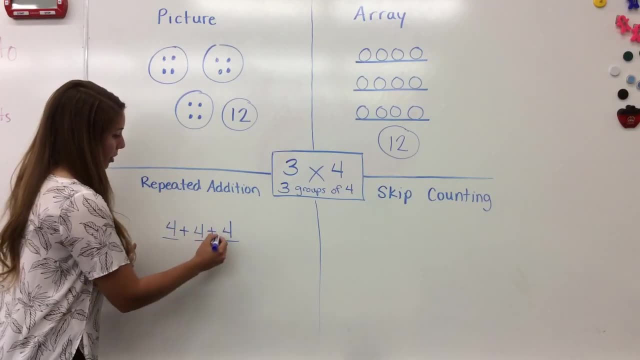 Now the name of this strategy is repeated addition, and what that means is I'm going to add the same number over and over and over. So I'm going to add these numbers up: Four plus four plus four, And that is going to give me my answer. 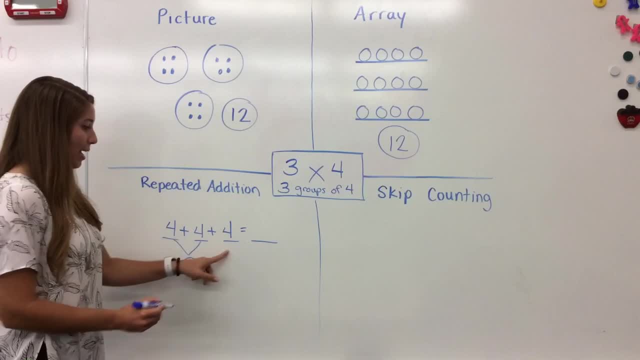 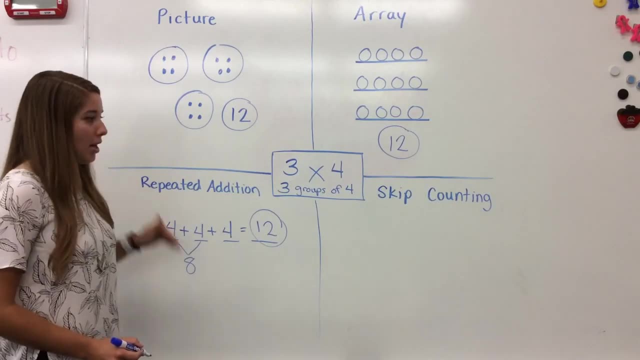 So when I add four plus four, I get eight, And eight plus four more equals twelve, And there's the answer to four times three using repeated addition. The last strategy, and the one you'll probably use the most, is skip counting. So when we skip count, we are going to count by one of these numbers. We can count by three or we can count by four. So if I'm going to count by three, I'm going to count four times by three, Three, six, nine, twelve.